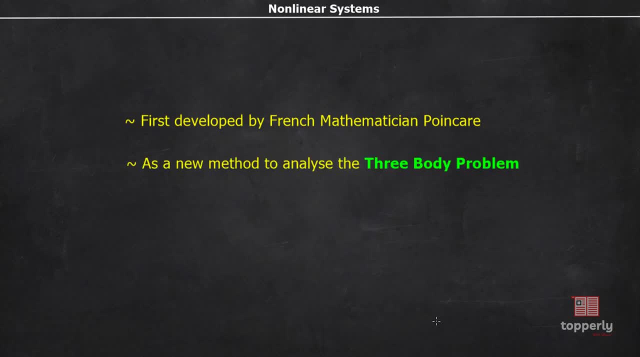 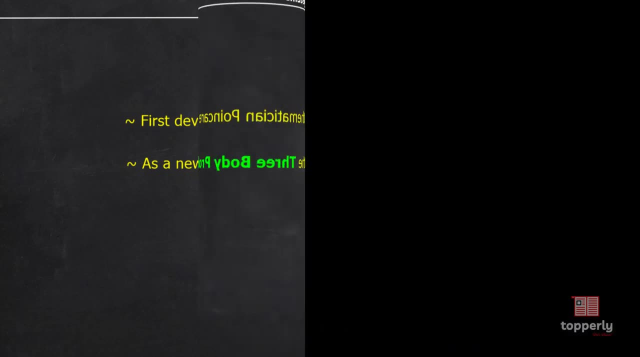 problem which defies Newtonian physics. Now, before going to the analysis part, we should know what is a phase plane For that. let's take an example of a simple paper. As students of engineering, we are all familiar with position time or velocity time graphs. Now 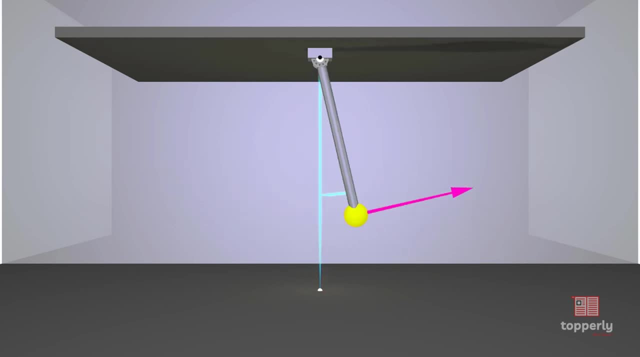 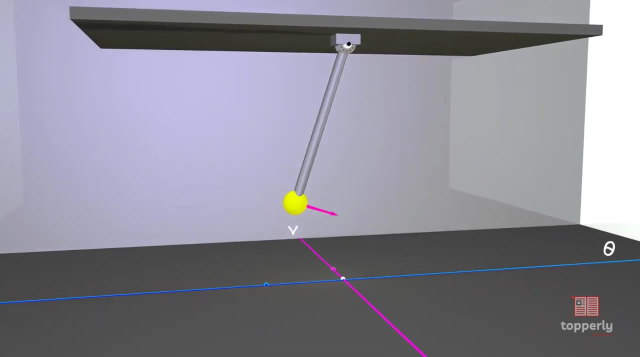 let's try to make a 2D plot that represents every possible state of the pendulum. On the x-axis of the graph we have the angle of the pendulum and on the y-axis we have its velocity. The resulting graph is called a phase: phase If the pendulum has friction. 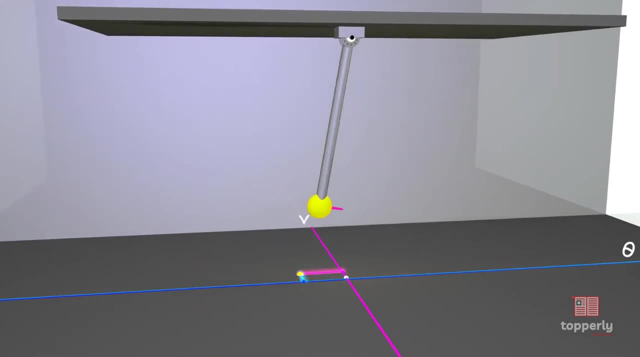 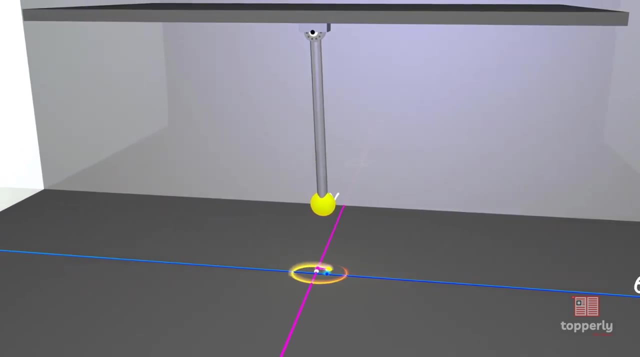 it will eventually slow down and the angle of the pendulum decreases with each swing. This can be seen in the phase phase as an inward spiral focusing towards the origin, which we know as an inverse spiral. Now let's look at the equilibrium state of the pendulum. No matter what the initial 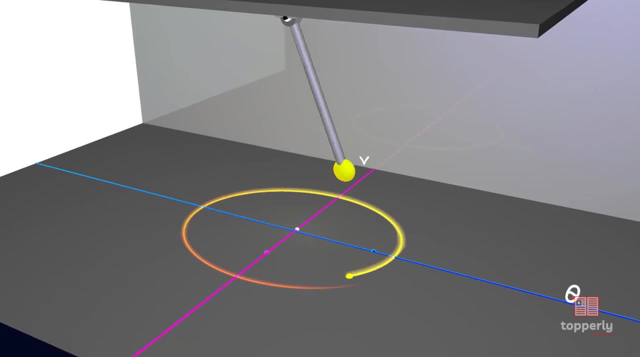 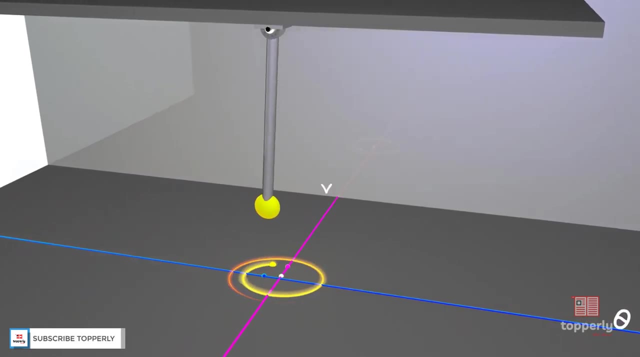 conditions are. if friction is present, we know that the final state of the pendulum will be at rest at origin, And in the graph you can see that the phase trajectory is attracted towards this equilibrium point. So this is called a stable equilibrium point. On the 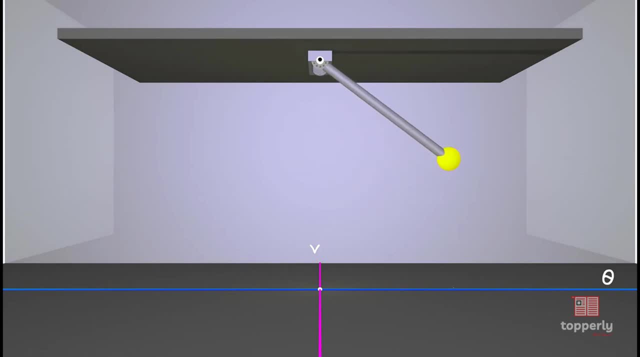 other hand, if friction is absent, then the pendulum does not lose energy and it will sustain its amplitude in every oscillation. This can be seen as a loop in the phase plane. These loops are called the equilibrium points. These loops are called the equilibrium points. 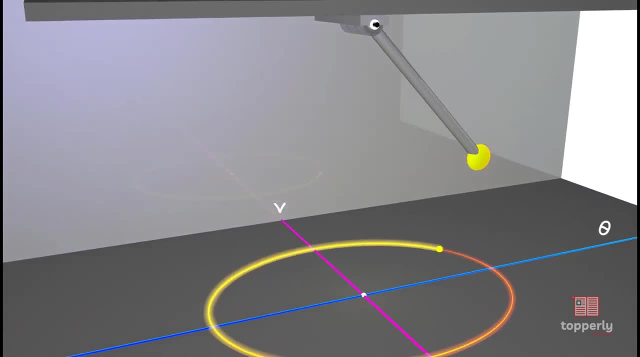 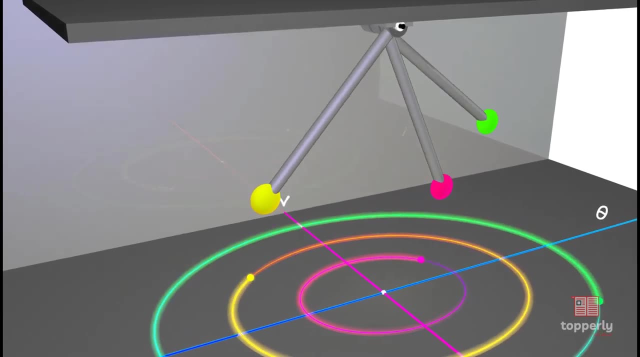 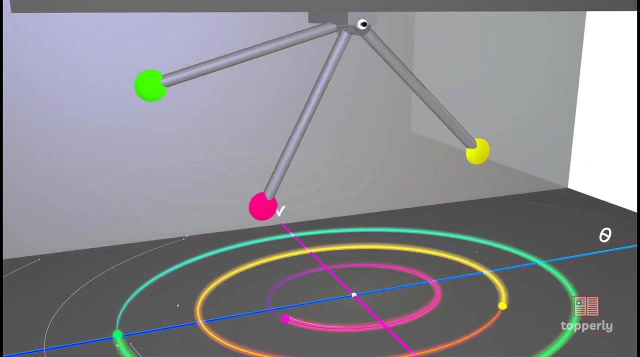 These loops are called limit cycles. We could swing the pendulum with different amplitudes, resulting in a very similar trajectory but different sized limit cycles. So when you see a limit cycle in state space, he can confidently say that the system is also having periodic, sustained oscillations. An important thing to notice is that the phase 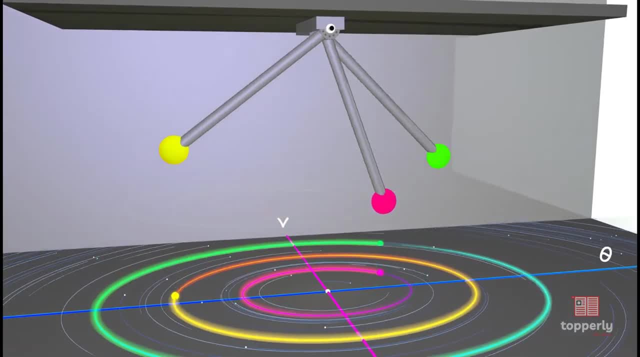 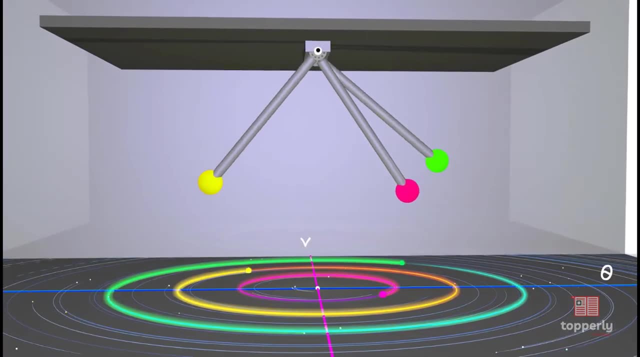 trajectories never cross each other in state space. This is because each point uniquely identifies the complete state of the system, and that state has only one future. So once, So once you choose an initial state, the entire future of the system can be theoretically determined. 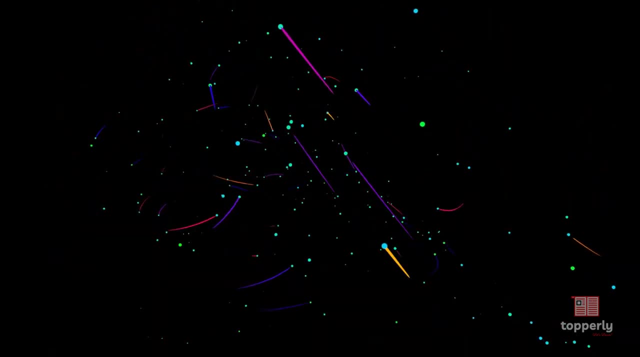 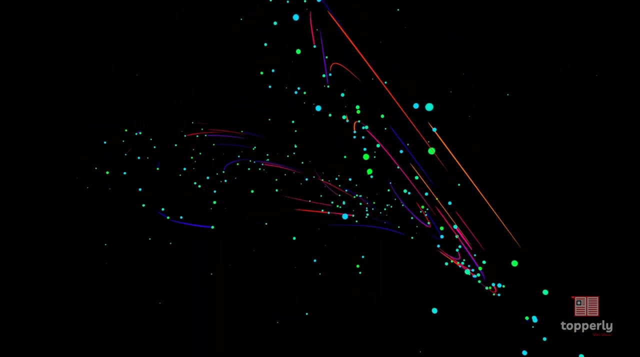 Now this same concept can be extended to higher dimensions, If you take the case of a 3D phase space. I am pretty sure that you all must have heard of the butterfly effect. At least you must have heard the famous statement of the butterfly effect. 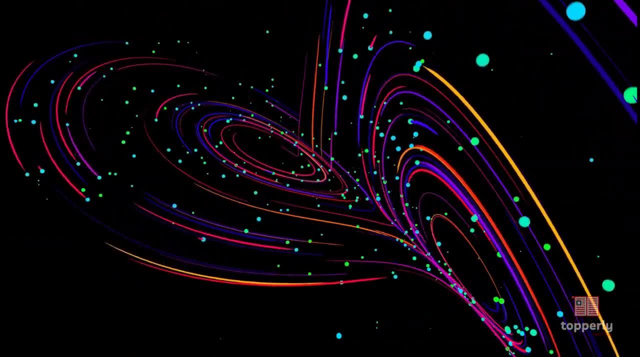 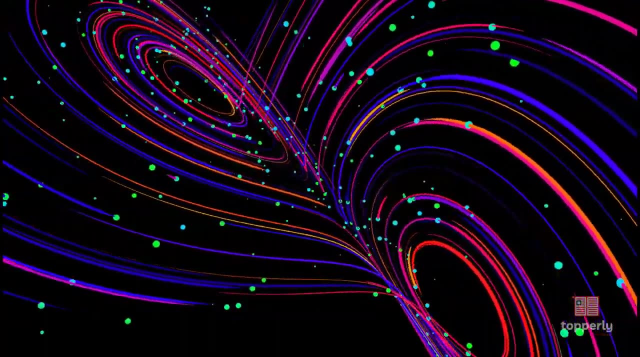 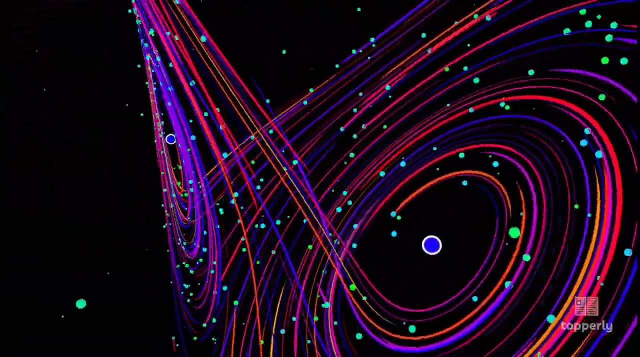 That is, a butterfly's wing flap in South America can cause a tornado in North America. The butterfly effect got its name not only because of this statement, but also due to this beautiful butterfly shaped phase trajectories it creates in a phase space. Now remember: all the paths traced out here never cross and they never connect to form a loop. 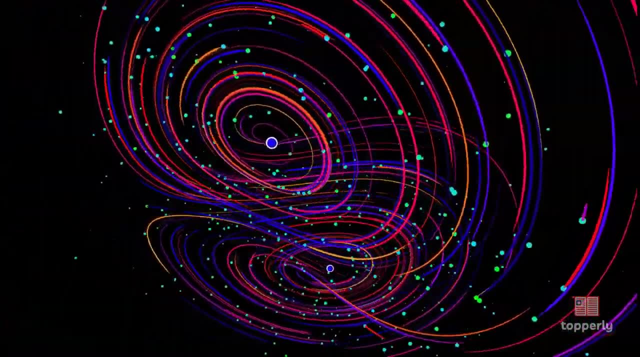 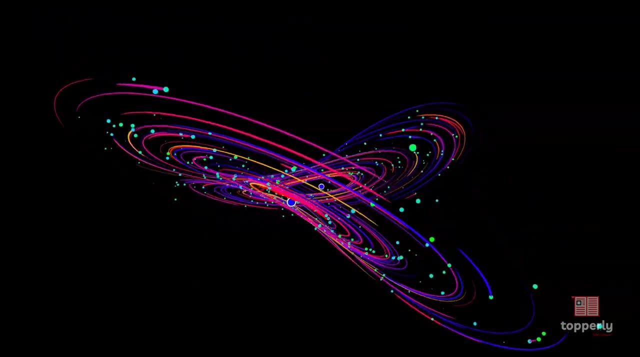 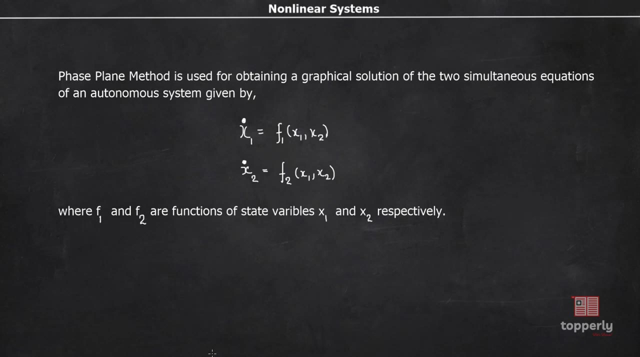 If they did, these loops are called limit cycles and they would continue on the loop forever and the behavior would be periodic and predictable. So I hope you got an idea about what a phase plane is Now defining. mathematically, phase plane method is used for obtaining a graphical solution for the two simultaneous equations of an autonomous system given by. 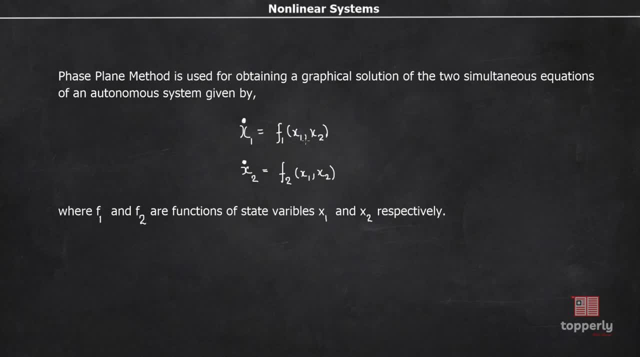 x1, dot equal to f1 of x1, x2,. x2, dot equal to f2 of x1, x2, where f1 and f2 are functions of state variables x1 and x2 respectively. Now, before concluding the lecture, let's go through a small theoretical topic. 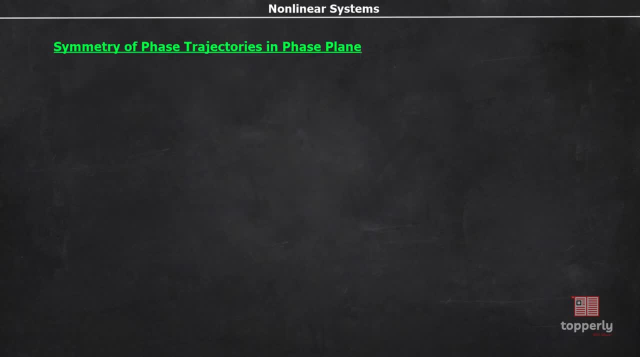 That is, Symmetry of states, Symmetry of phase trajectories in phase plane. First we will talk about the symmetry of the phase trajectories about x1 axis. For that let's take a differential equation given by y double dot plus f of y comma, y dot equal to 0.. 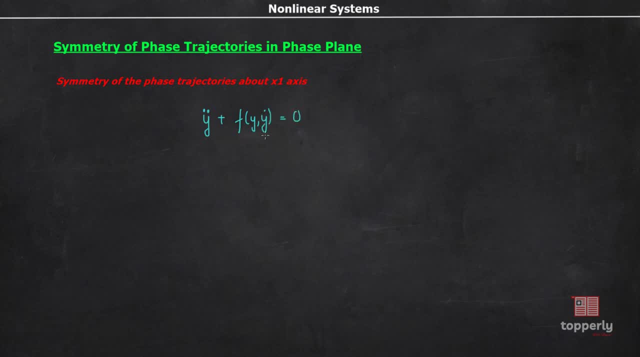 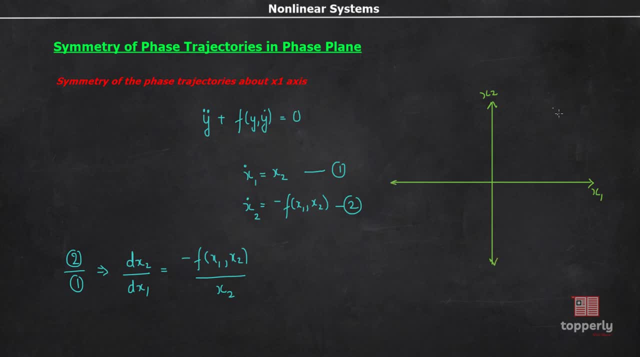 f of x1 comma x2- dot equal to minus of f of x1 comma x2- dot equal to minus of f of x1 comma x2.. For simplicity, let us assume the function f of x1- x2 as a straight line passing through origin. 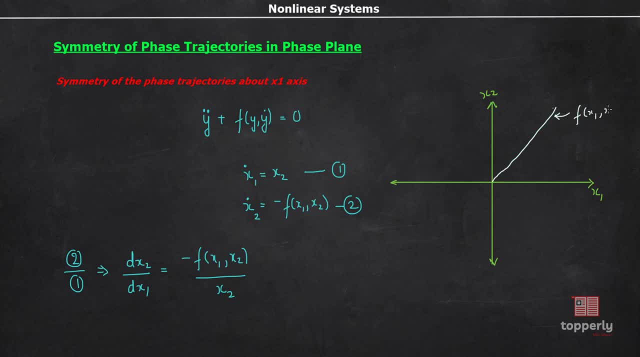 So this is f of x1 comma x2.. Now, mirroring this function about x1 axis, we get a graph like this, and this graph is given by f because this is minus x2 axis. Now, taking the slope of this function, we get it as dx2 by dx1, equal to minus of f of x1,x2. 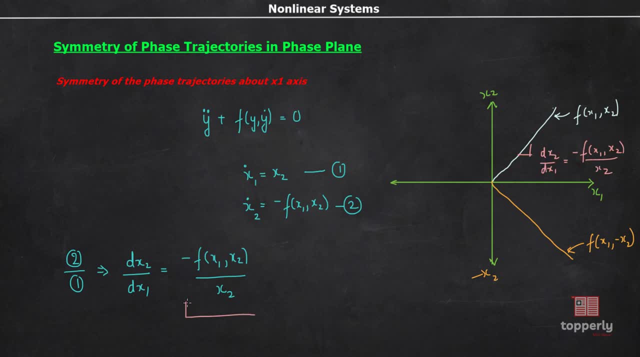 by x2.. We have obtained that over here. Now, taking the slope of this graph, dx2 by dx1, equal to minus of f of x1, minus x2 by x2.. This minus is because we are taking about negative x2 axis. 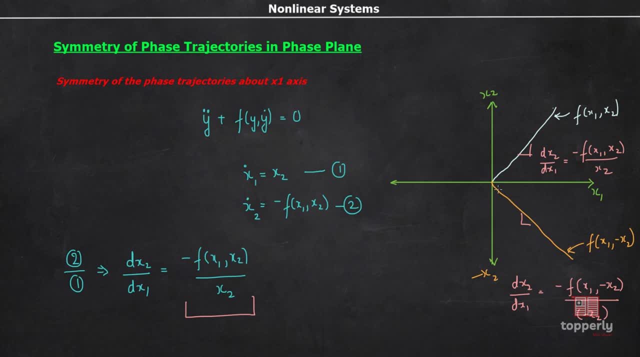 Now by observation we can see that the slope of these two trajectories should be equal in magnitude but opposite in sign. That is, if the slope of this one is theta, then the slope of this one should be minus theta. For this condition to be satisfied here, f of x1,x2 should be equal to f of x1, minus. 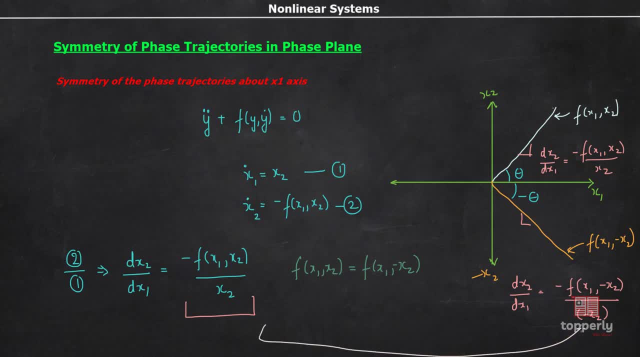 x2.. Let me show you why. For that, let us write this down again: dx2 by dx1 equal to minus of f of x1, minus x2 by minus x2.. Now, since f of x1, minus x2 is equal to f of x1,x2, we can write this down as minus of: 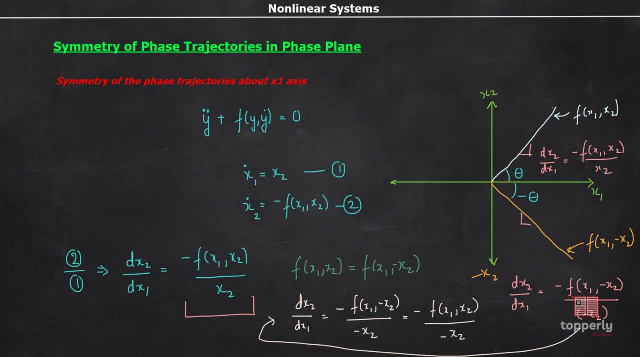 f of x1,x2 by minus x2.. Now If I write this equal to p, then you can see that this much part is equal to p. therefore this equation becomes minus p. Therefore, the condition that the slopes must be equal in magnitude but opposite in sign. 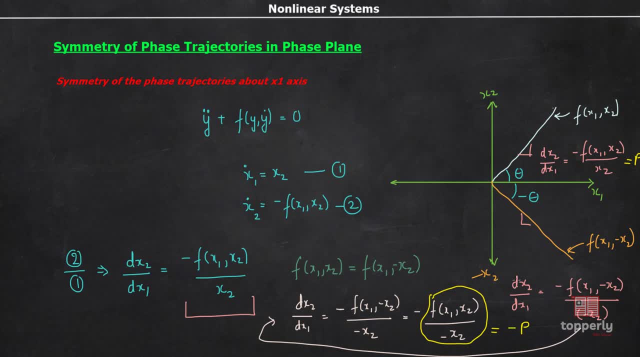 for x2 greater than 0 and x2 less than 0 is satisfied. Thus we can conclude that for these trajectories to be symmetrical about the x1 axis, the condition is the function f of x1,x2 must be equal to f of x1,x2..